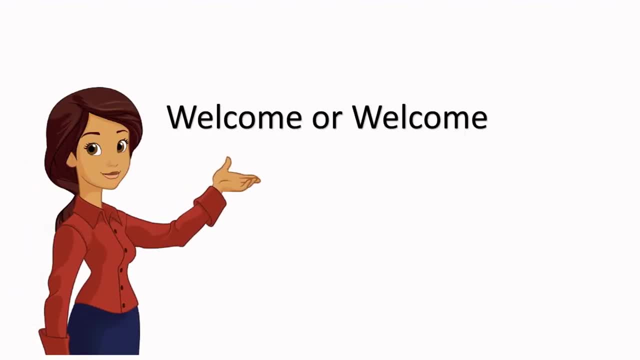 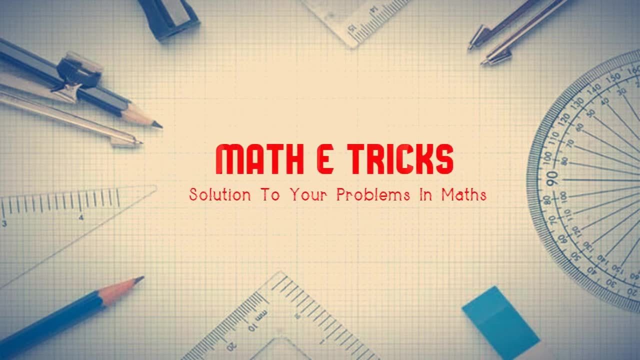 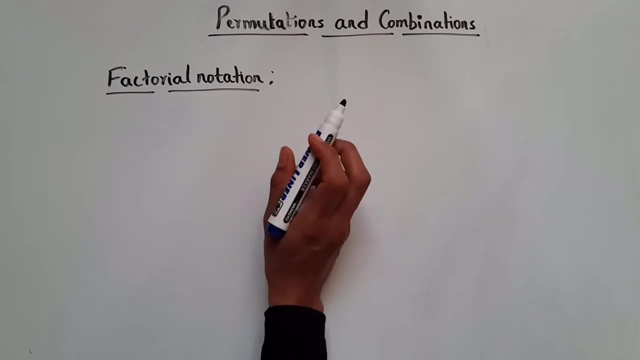 Hi guys, welcome, or welcome back to my channel. In this video we will see what is factorial notation. In my previous video we have seen fundamental principle of counting, So if you haven't watched that, there is a link in the description box below. you can check that out. So here in order to learn permutations. 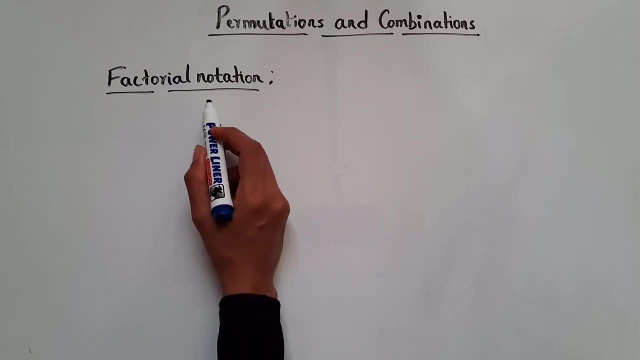 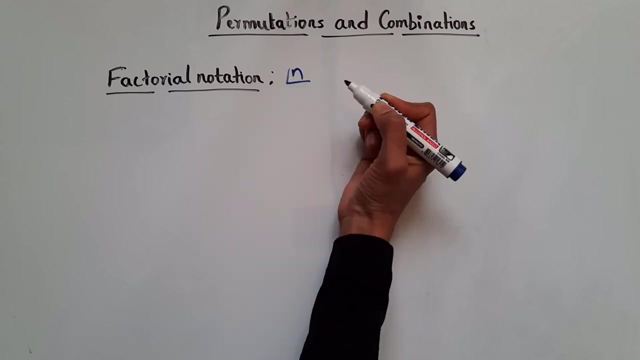 and combinations. first we need to know what is factorial notation or factorial of a number. We will be using this in permutations and combinations. So what is factorial notation or a factorial of a number? So it is denoted as n factorial or it can also be written as: 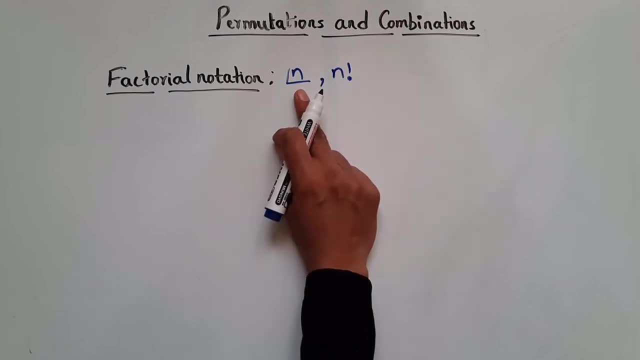 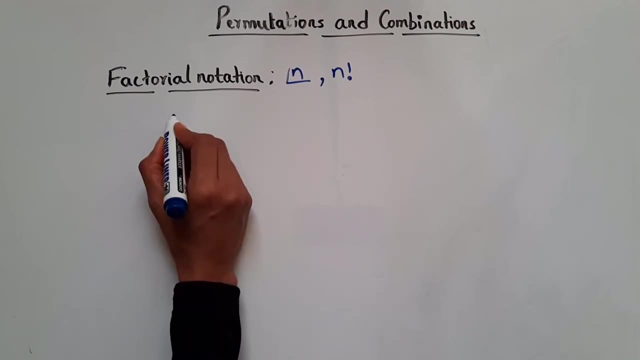 n factorial. So here n is a positive number. So factorial notation is defined only for the positive numbers. Alright, Let's say we have 5 factorial. What is the value of 5 factorial? So 5 factorial is nothing. 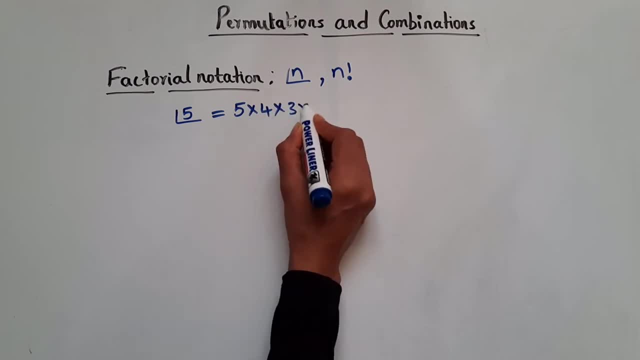 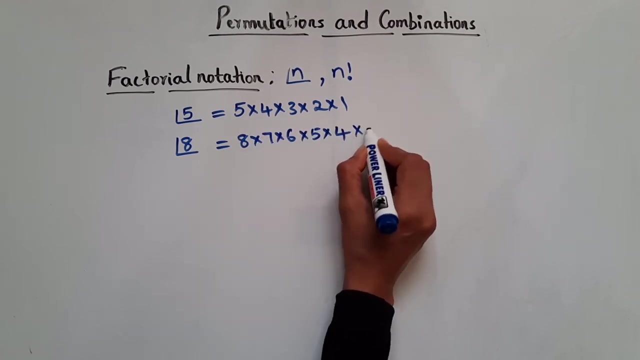 but 5 into 4, into 3, into 2, into 1.. Let's take any number. Let's say we have 8 factorial, So it will start with 8 into 7, into 6, into 5, into 4, into 3, into 2, into 1.. Now let's. 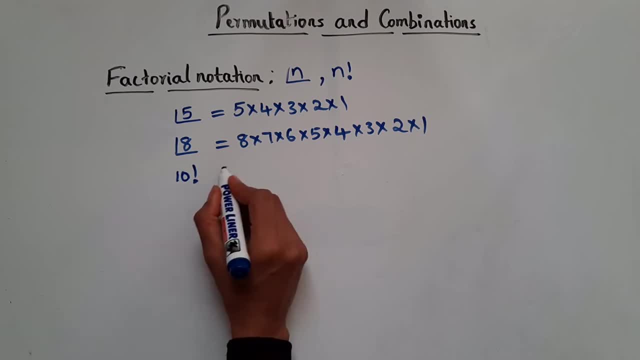 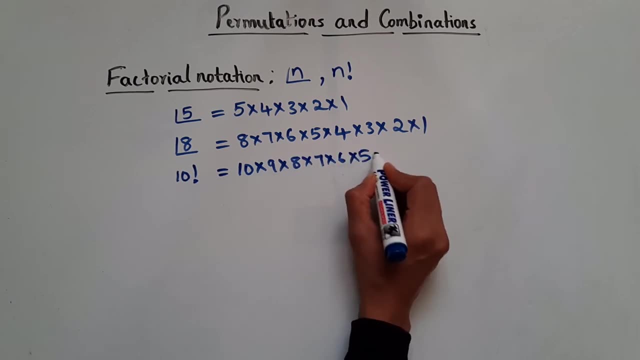 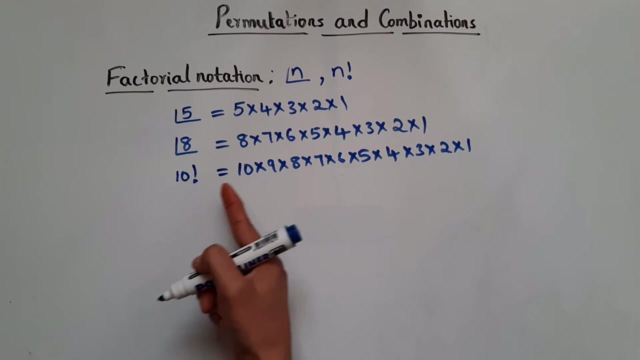 see what is 10 factorial. We can write like this also: It is equal to 10, into 9, into 8, into 7, into 6, into 5, into 4, into 3, into 2, into 1.. So this is how you will find the factorial of a number. So in: 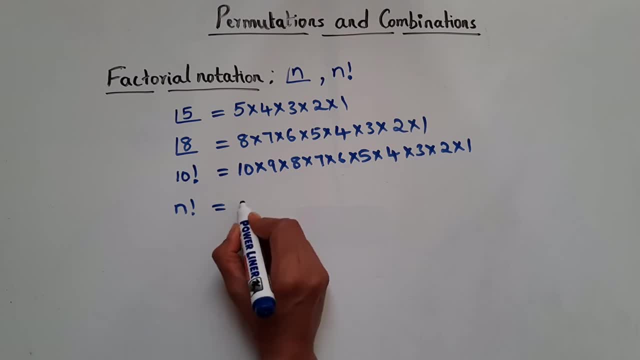 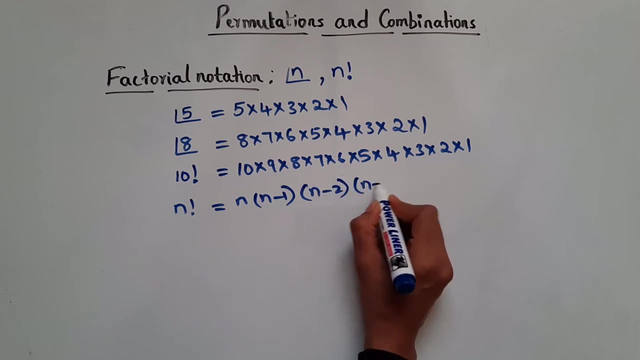 general what I can write. n factorial is equal to n into n minus 1, into n minus 2, n minus 3, and so on up till 3 into 2 into 1.. Right, So this will be the general form to write. 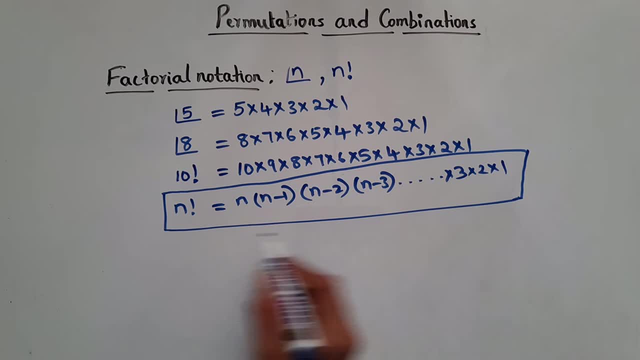 the factorial of a number. So if n is 10.. So 10 into 10 minus 1 is 9.. Similarly, 10 minus 2 is 8, and so on up till 3 to 1.. Right Now, same equation. can I write this as n factorial? 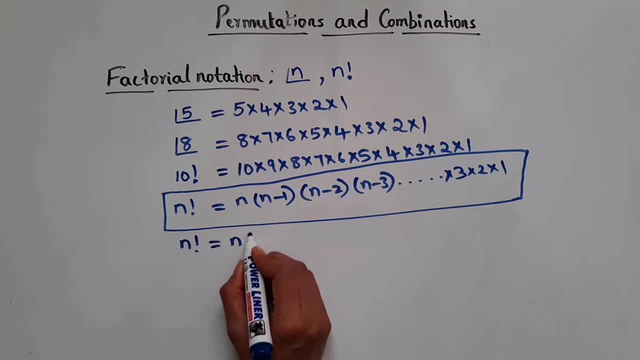 is equal to n factorial Right. So this is how you can write it. So this is how you equal to n into n minus 1 factorial, So n. I wrote as it is. So this is what n minus. 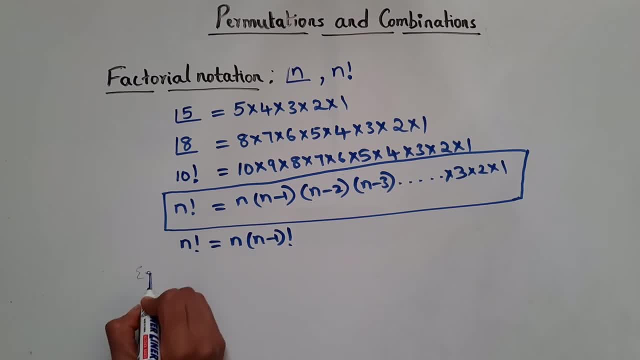 1 factorial right. If I were to give example here, if I take 5 factorial, we have 5 into 4, into 3, into 2, into 1.. So can I write this as 5 into this is 4 factorial. What is 4? 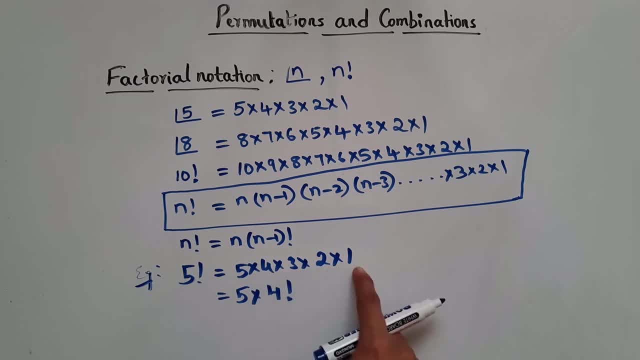 factorial 4 factorial is 4 into 3 into 2 into 1.. So I can replace this whole thing as 4 factorial, right? So we have a property called as n. factorial is equal to n into n minus 1 factorial. So you can write: n. factorial is equal to n into n minus 1 factorial. Now 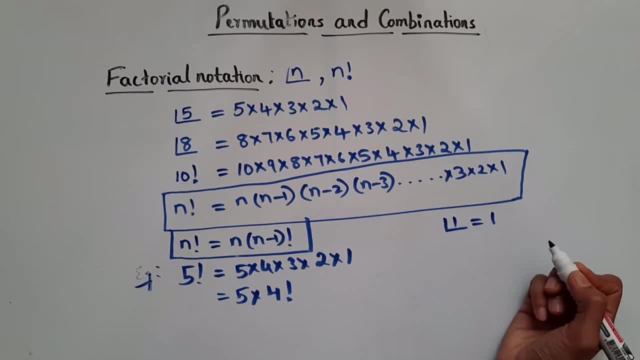 what is 1 factorial? 1 factorial is 1.. What is 0 factorial? 0 factorial is also 1.. How 0 factorial is equal to 1?? Let us say we have 1 factorial is equal to, if I put: 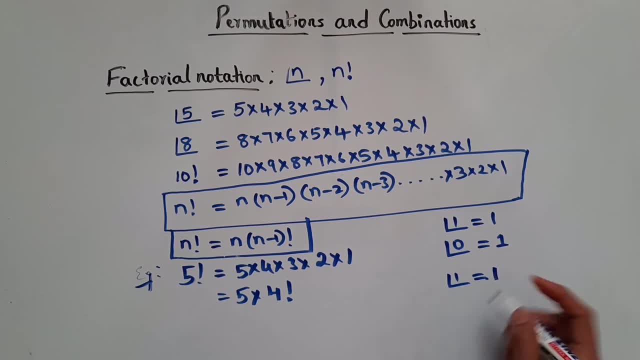 this property, so n is 1, 1 into n minus 1.. So 1 minus 1 is 0.. So 0 factorial, right. So I can write 0 factorial. So from here 0 factorial is what Factorial of 1 is 1. 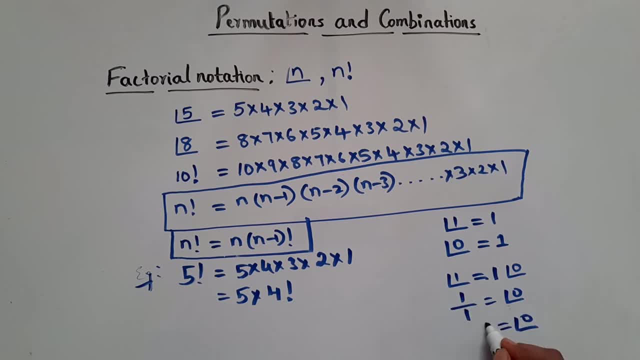 by 1.. So we can say: 0 factorial is equal to 1 factorial. So always remember this: 1 factorial is 1 and 0 factorial is also 1.. Alright, I hope this is clear. Now let us see problems based on this. But before that, pause the video. 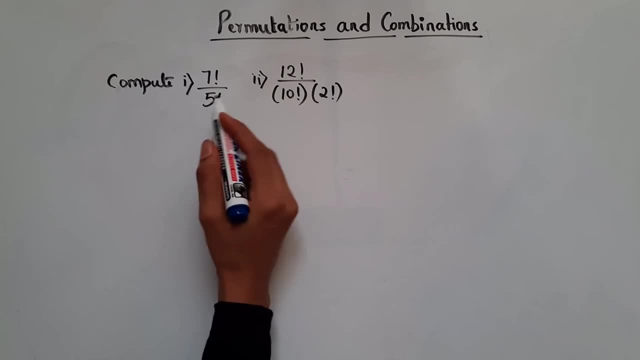 and note this down. So we have compute 7 factorial by 5 factorial. So what is 7 factorial by 5 factorial? So 7 factorial, that is 7 into 6 into. can I write 5 factorial Right By this 5 factorial? 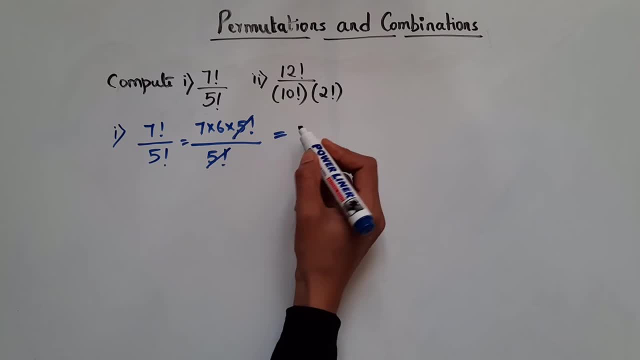 I can cut this. What is 7, 6 r, 42. Here 5 factorial is nothing but what? 5 into 4, into 3, into 2, into 1, right? So since I have 5 factorial, I can cut them. So I wrote it. 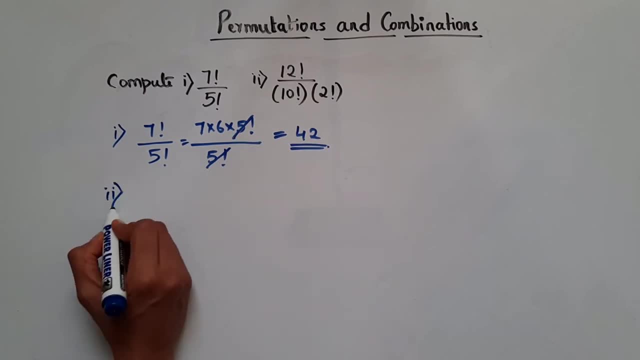 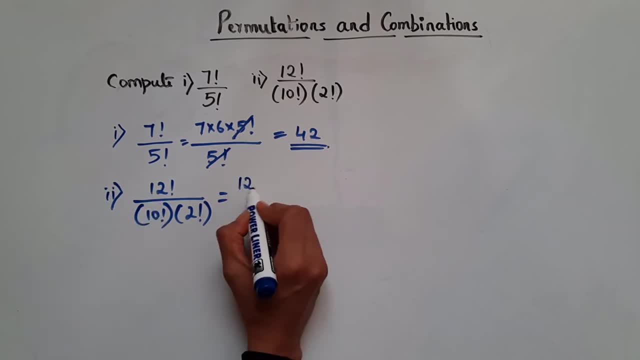 5 factorial by 5 factorial, So we have 5 factorial by 5 factorial, So we have 5 factorial by factorial. what I can write here, So 12 into 11, into 10 factorial, right by this 10 factorial. 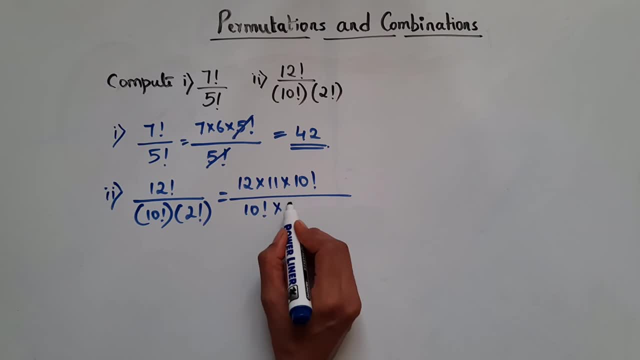 I will keep as it is, So I can cut them into 2 into 1.. 2 factorial is 2 into 1.. So this and this is gone, We have 2. ones are 2, 6 are 12.. So here, this is 6 into 11 is 66. Now. 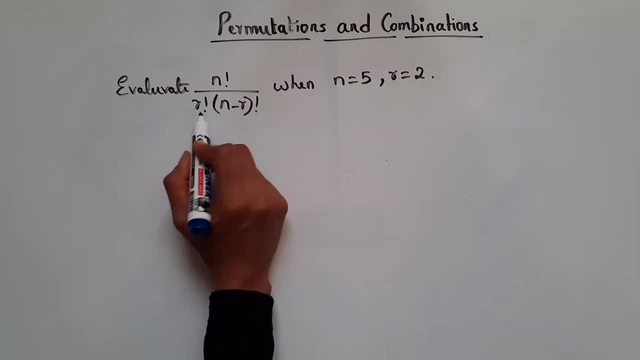 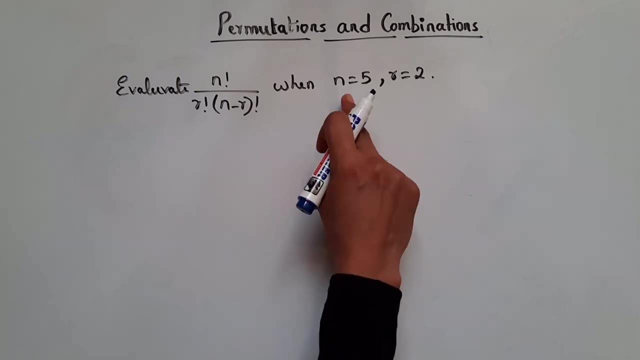 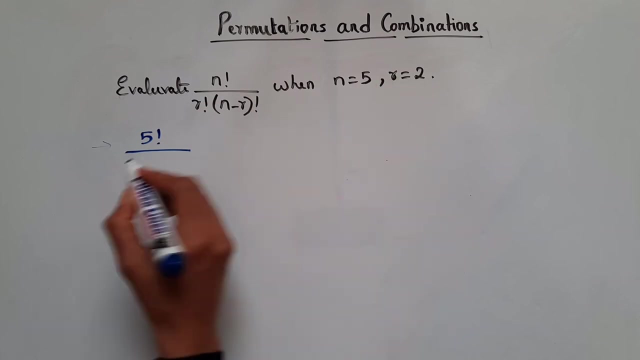 let us see the next one We have. evaluate n factorial by r factorial into n minus r factorial, when n is equal to 5 and r is equal to 2.. So let us substitute the value of n and r in this, So we have n factorial, that is 5. factorial by r is 2.. So 2 factorial. 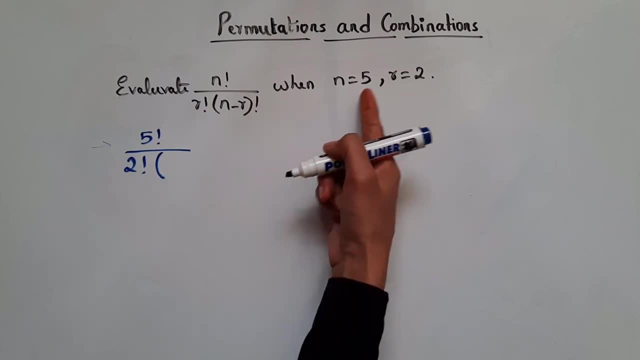 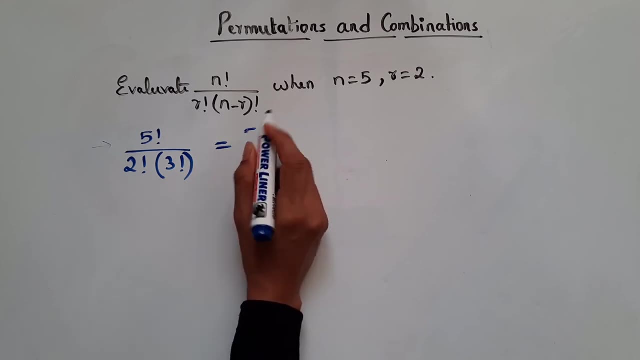 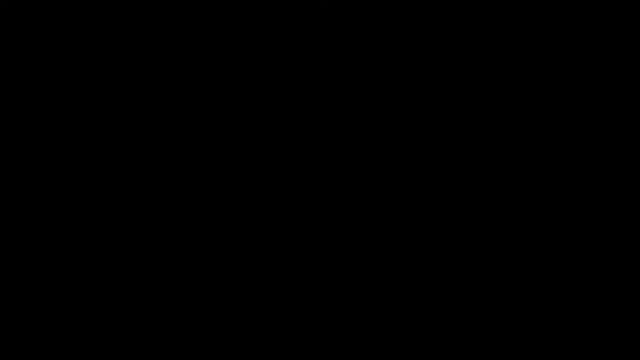 into n minus r, 5 minus 2 is 3.. So 3 factorial, which is equal to. So we have 5 factorial. What is 5 factorial? 5 factorial is nothing but 5 into 4, into 3 factorial, right by. So here we have 2 factorial. 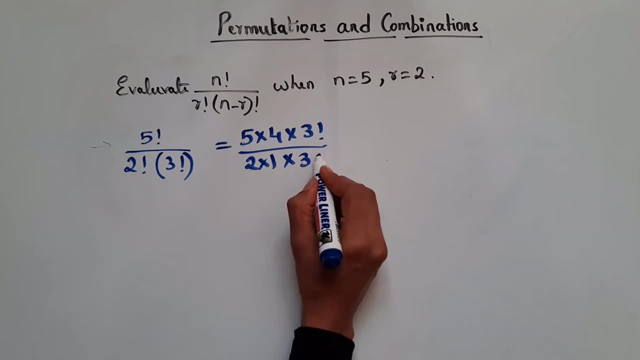 So 2 into 1, into this 3 factorial keep as it is, So I can cut here right. So 2 ones are 2, twos are 4.. So 5, twos are 10.. Now let us see one last problem. So let us see this: 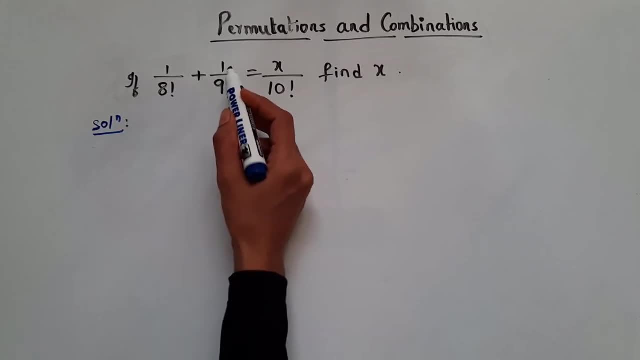 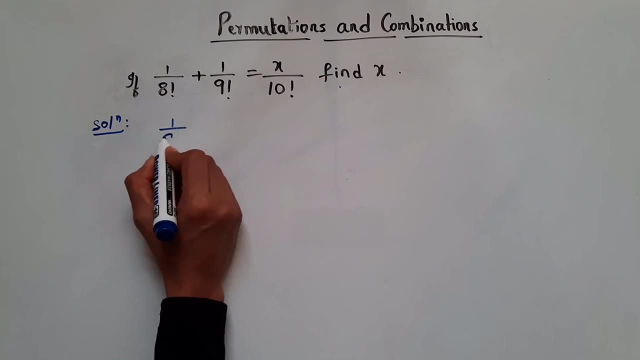 last problem. Here it says: if 1 by 8 factorial plus 1 by 9 factorial, So we have 1 by 8 factorial is equal to x by 10 factorial, Find the value of x. So we have: 1 by 8 factorial plus 1 by 9 factorial is equal to x by 10 factorial. So this implies: